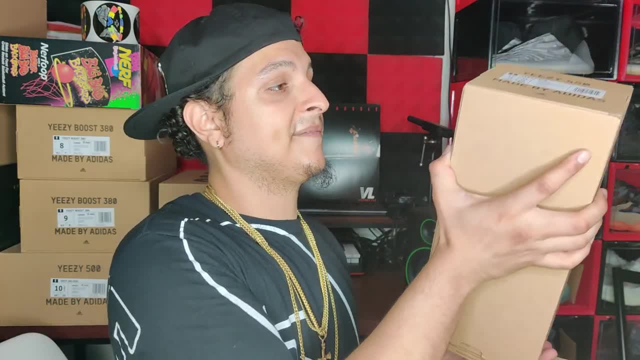 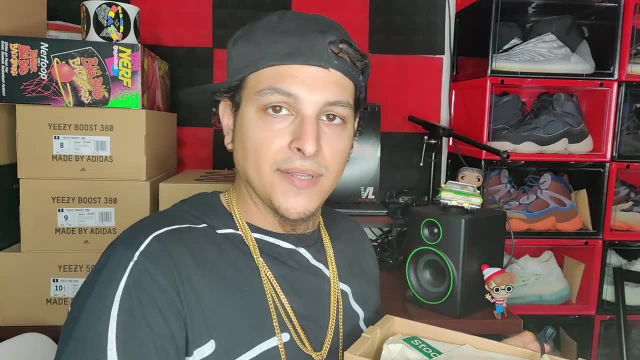 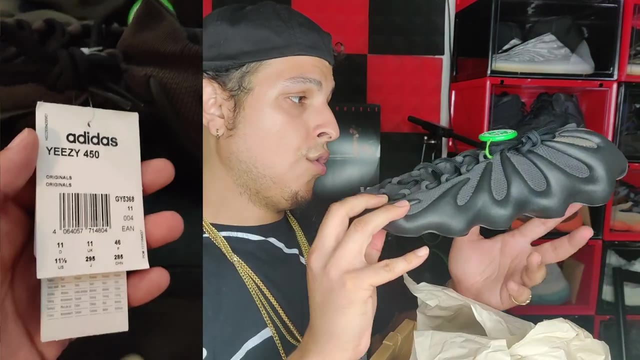 going to let you guys know if that was the right decision. I think it was. That's my guess That it was a good decision. StockX, StockX. I'll be showing you the tag in a second. guys, Don't worry, I'll probably put the tag on the side of this video. Yeah, New sticker. 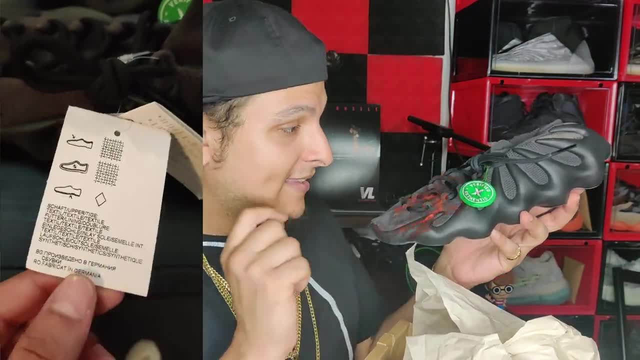 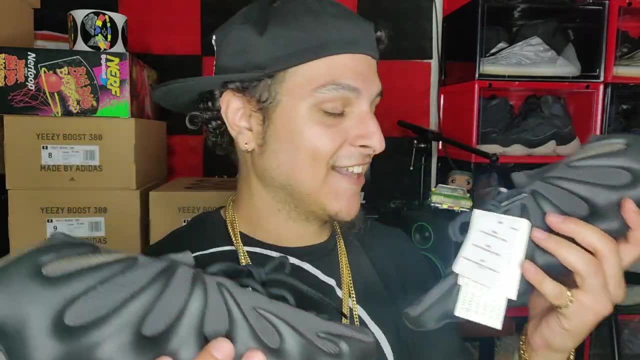 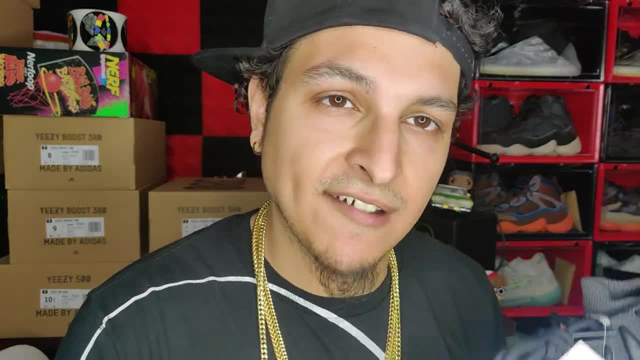 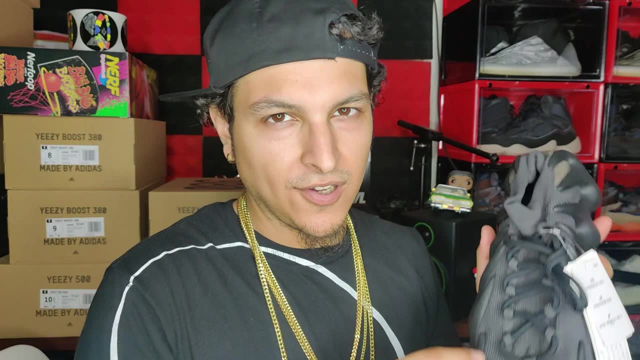 this collection. Yeah, You're in trouble. You're in trouble, boy. I just let you guys know because I've been seeing so many reviews on this before you know, prior to this, This package shipment And I got to say, while this upper looks really bright compared to, 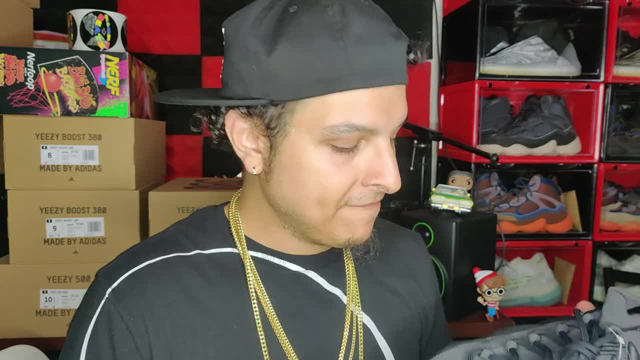 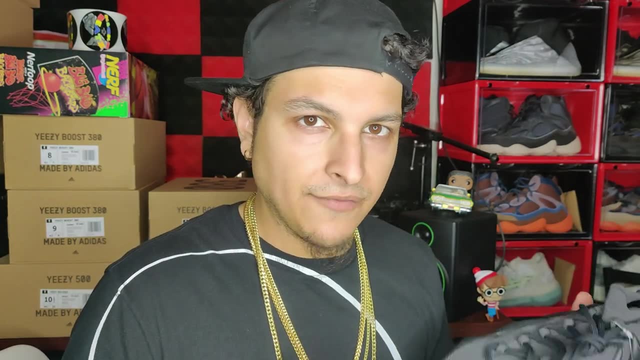 the midsole in these videos like. it looks like a light gray of some sort. That's not how it's going to appear to you. when you receive this in person it will look a lot darker, But the reason why it just has that look to it in videos and photos is because it is tech-based. 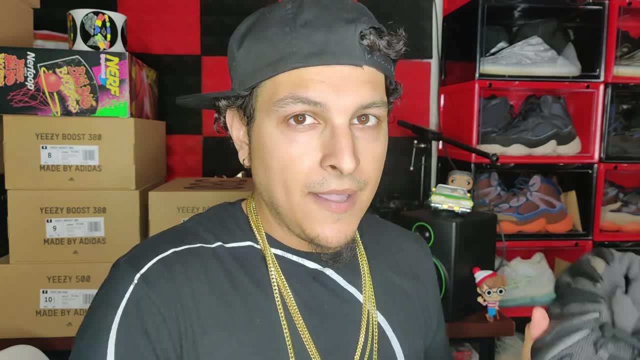 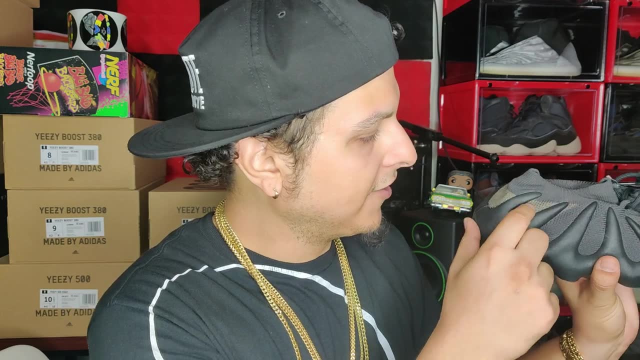 it is technically brighter than the midsole, but it will appear a lot darker in person. just take my word for it, guys, it really will. there is a color difference in the back here. this coloring you see here is obviously different than the rest of the shoe. for the upper and midsole it's more. 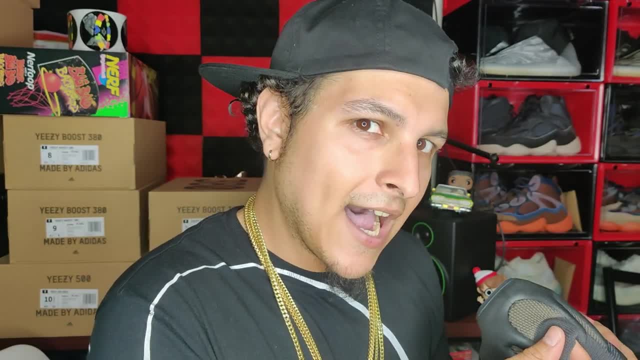 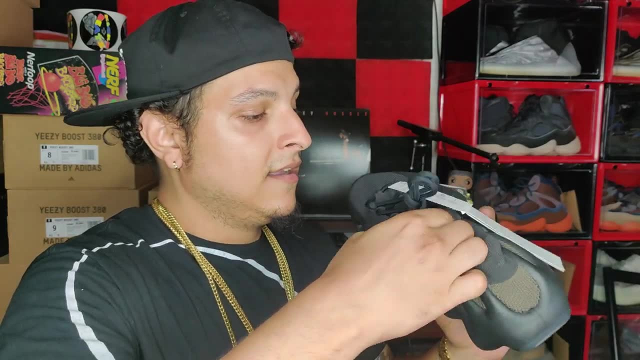 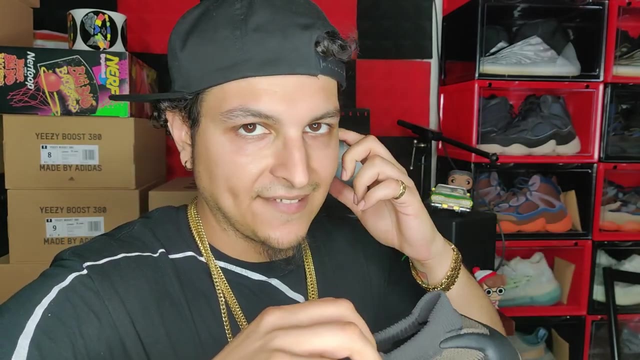 like on the. i want to say kind of like olive greenish, grayish. yeah, it's like a special olive green of some sort that he chose for this backside, definitely, and of course guys, this feels sock like on the upper right here around the ankle area. i like how it feels. it's not as tight as the. 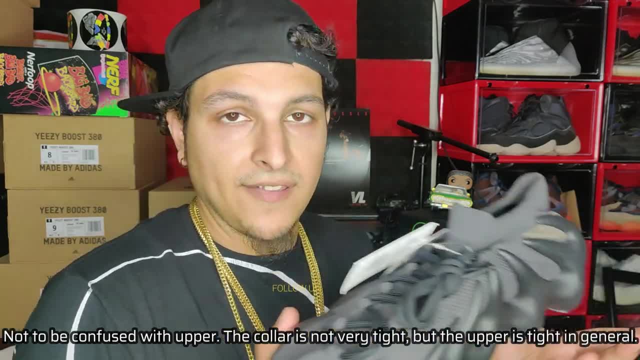 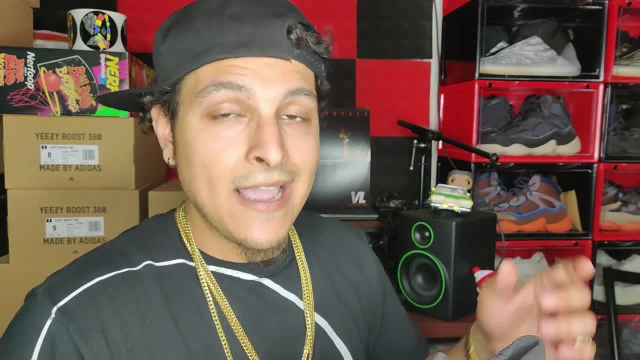 yeezy 380, that's for sure. and uh, yeah, we're gonna try this on feet. let you guys know, um, how i felt about going to full size up. like i said, and for those thinking about resale right now, now is the perfect time to get this, seeing that it's going for around 280 average via stock x. before clicking: that buy now button and seeing the extra charges applied, of course, it's averaging around 280. it was higher than that just two weeks ago, so i'd say, do that. why are the prices dropping? i think it's because of a restock. there's definitely going to.